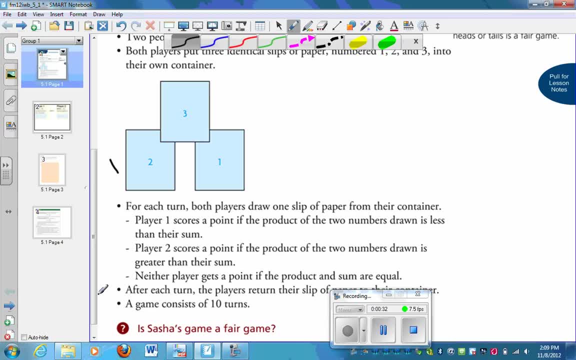 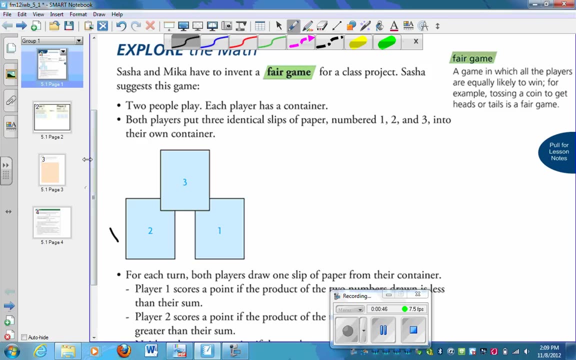 Player two scores if the product of the numbers is greater than their sum and neither if they're equal. Ten turns is a game. After each turn they return all the slips. Is it fair? And this is how we define fair, And everyone has an idea of what fair is. In math we say a game in which all the players are equally likely to win, For example, tossing a coin. So I know people like to say: well, fair isn't the same as equal. In math it is. I'm not trying to tell you. 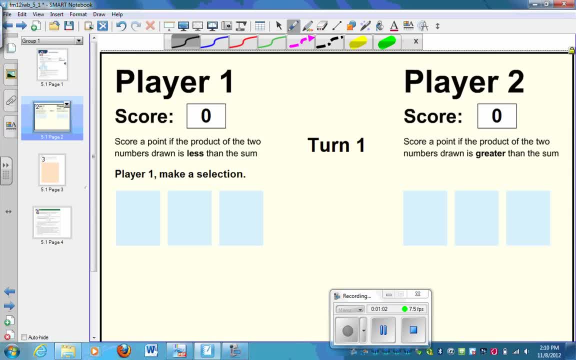 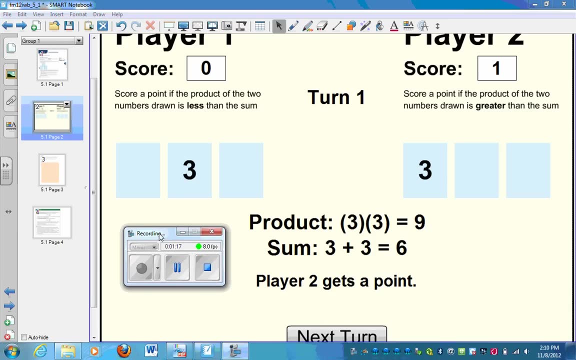 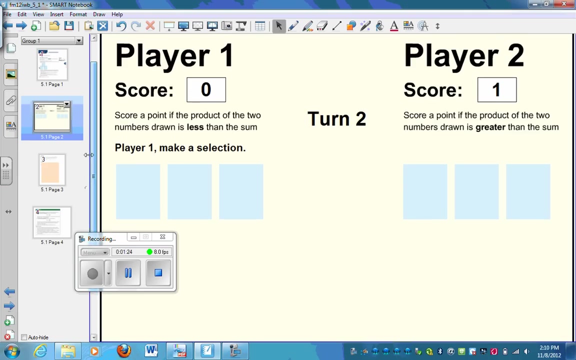 in the real world, but we're talking in the math world, which, I mean, is still real, Anyways. so let's see: Player one chooses and they get a three. Player two chooses and they get their three. The sum is nine, The six, the product is nine, So player two gets a point. You see that right there. Let's play again. Okay, Player one chooses, I get two. This person gets one, So the product is two, The sum is nine. 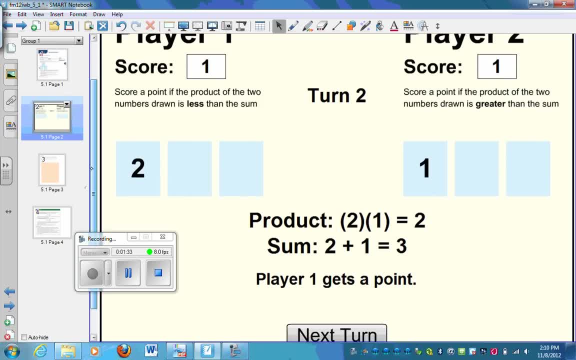 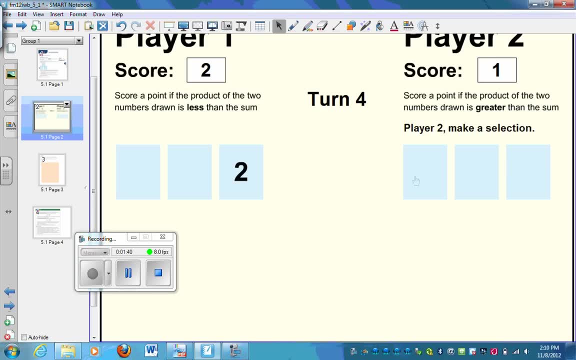 The sum is three. Player one gets a point, A one and a three. Player one gets a point. again A two and a one. Again player one. Well, is this feeling pretty fair? Two and a three? Nope, Two and a three was good for player two. Player one gets a point. 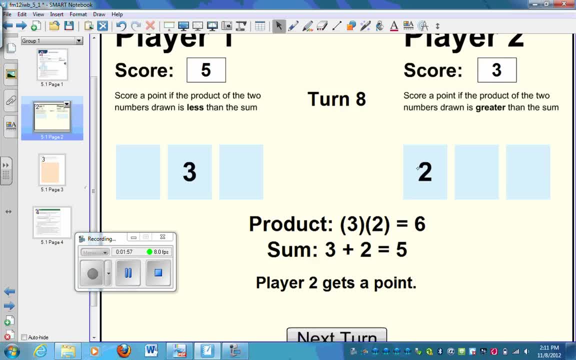 Player one gets a point. Three and a two. Yes, Player two. Three and a two. Good, Two and a two. It's a draw. No points. Remember if they were the same: Three and a two. Player two gets a point. Oh, I started over already. 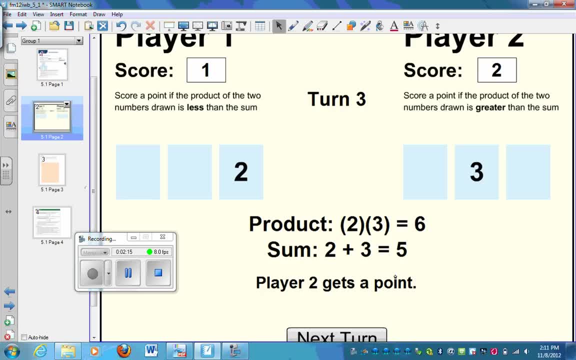 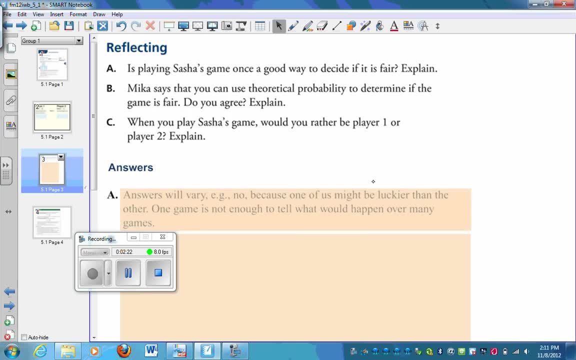 Anyways, you can see that player one seems to be getting a little more points than player two. in general, Is playing it once a good way to decide? Well, no, because one of us might be luckier than the other. Mike says that you can use theoretical probability to determine. 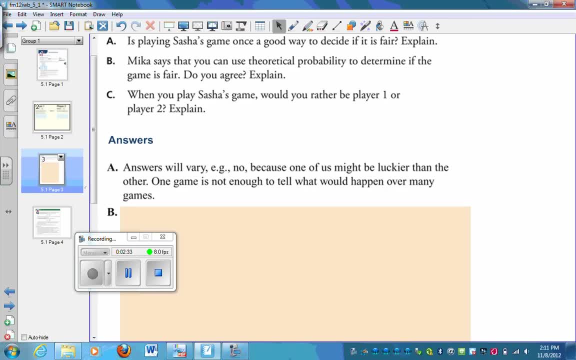 if the game is fair, Do you agree? So theoretical is saying: okay, this is what should happen, This is theoretically what can happen. In theory, all the ways that player one can win player one is if the product is less than the sum. 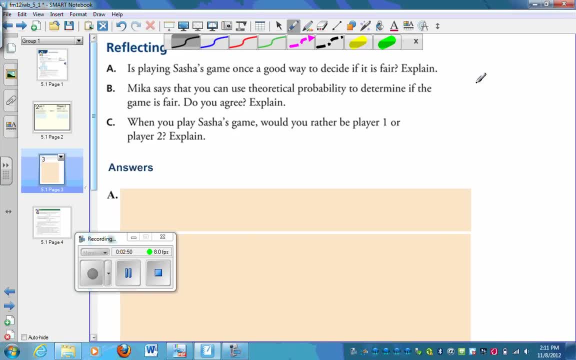 all the ways that that can happen are if we have a one and a two, or if we have a two and a one, Okay, Okay, Okay. And then if we get a three or a two and a three, or a two- oops, sorry- or a two and a three. 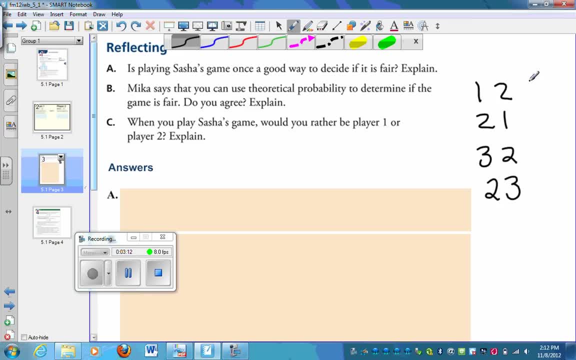 this is the case where player two wins. But what if we get a one and a three, or a three and a one? Player one wins. So these are all the ways player one can win and these are all the ways player two can win. 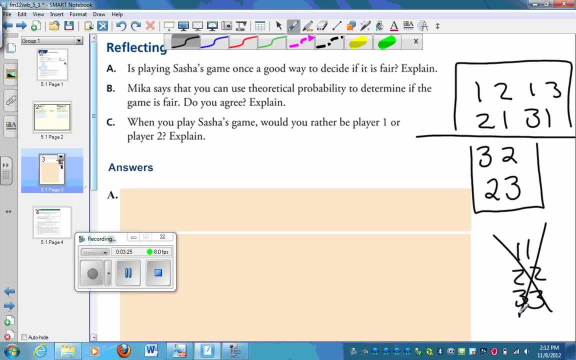 Remember, if we get these cases, nobody wins, Everybody loses. So theoretically, it seems like this is going to be more often, But when you actually go through an experiment, that's not always the case. that's going to happen More often. this should happen, but that's not the way it works. 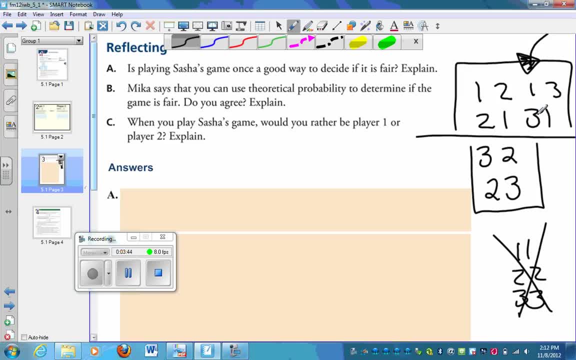 Theoretically, none of us should win the lottery, right? The odds are awful, But someone does. okay, When you play Sasha game, I'd rather be player number one, because that's about who wins more. Okay, just to summarize. 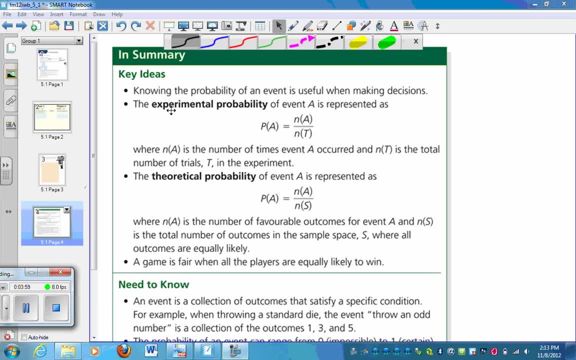 knowing the probability of event is useful in making decisions. Experimental probability is given. the probability of A is equal to the number A, the number of times that occurs, divided by And. NT is the total number of trials in the experiment. So probability of A is how many times A happens over the total amount. 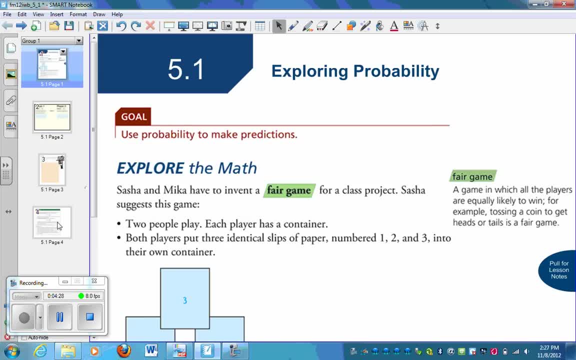 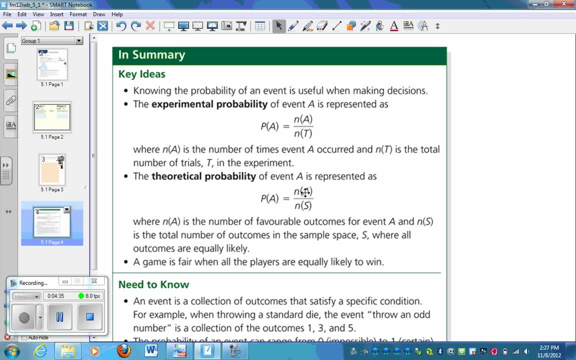 So what we were looking at is how many times does one win over the total and how many times does one lose over the total? So that's experimental, Theoretical says: okay, theoretically, what is the probability of A, The number of favorable outcomes? 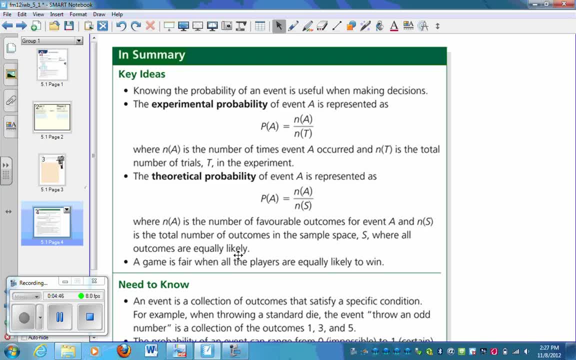 and this is the total in the sample space where all outcomes are equal. So sample space is all the possibilities. So there is a way that theoretically, all the possibilities is not what's going to actually happen when you play. There is a difference.